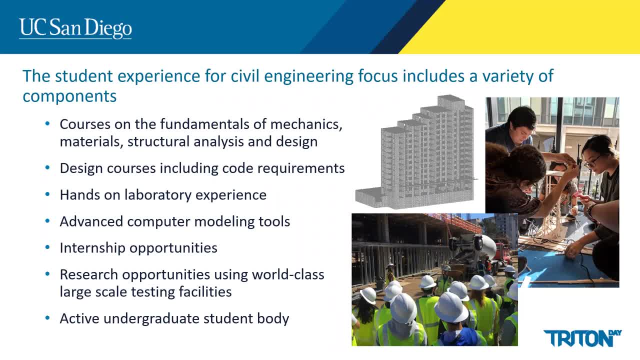 The student experience at UC San Diego is composed of several components, including courses on the fundamentals of mechanics, materials, structure analysis and design. We also have a series of design courses in which students learn the core requirements and how to detail steel, concrete, wood and other types of members for design. We have a series of laboratory. 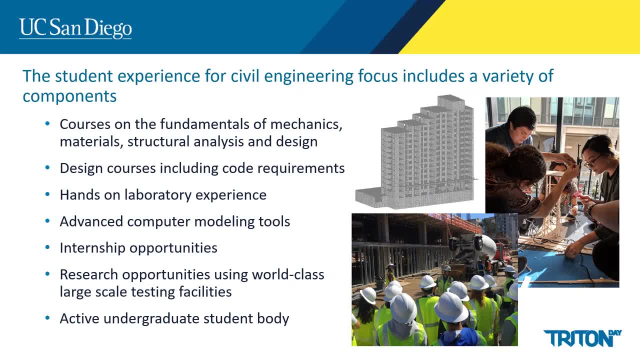 experiences that are part of many of our classes. We also use advanced computer modeling tools such as finite element simulations, And students also have the opportunity to get involved with internship opportunities or research with faculty through the summer or the academic year. Our students are also highly active in many student organizations. 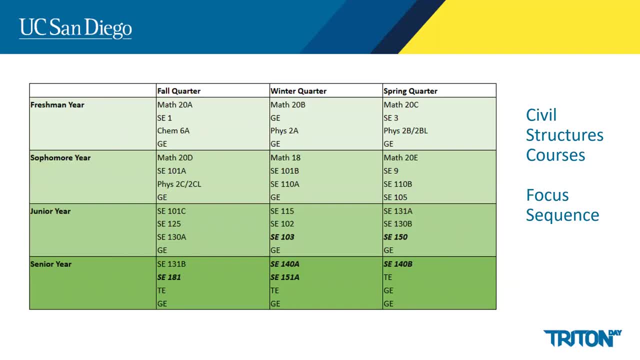 You can find more information on our course requirements on our department website. However, I wanted to provide a brief overview of the course. Students selected in the civil structures focus sequence will take four courses. The capstone course sequence and technical elect is all shown in bold here. 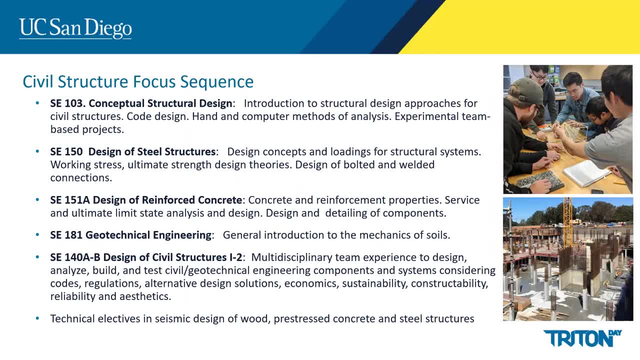 The courses include conceptual structural design, an introduction to structural design approaches for civil structures, including hand and computer method of analysis based on experimental team projects. Students will also take a class in steel structures showing the design concepts and loading for structural systems. how to design the members as well. 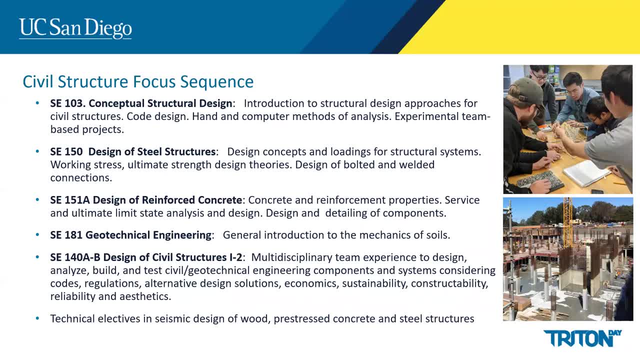 as how to connect them through bolted or welded connections. In the design of reinforced concrete, students will learn about the properties of concrete and the steel reinforcement, how to design the members and detail the components to sustain loads. We also take a class in 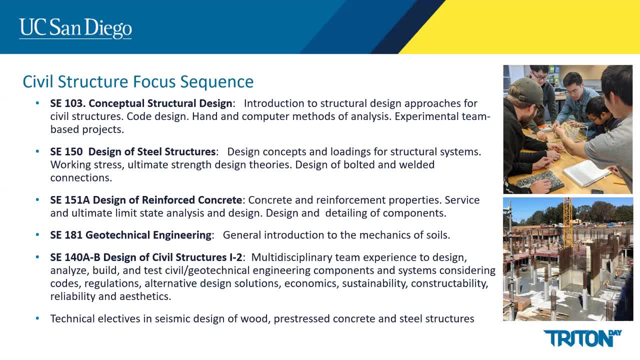 geotechnical engineering to learn more about the supporting soil in the foundation, And students will then be prepared to take our capstone sequence, which is design of civil structures, in which a multidisciplinary team of students will design, analyze, build. 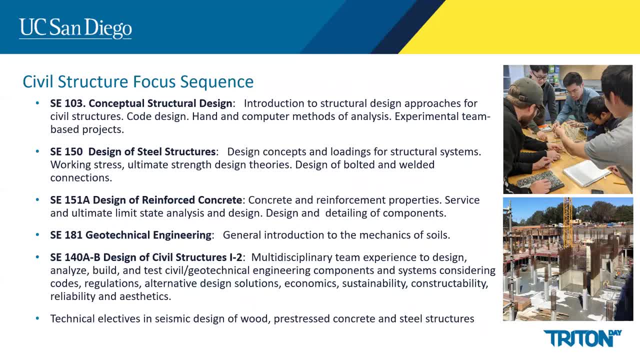 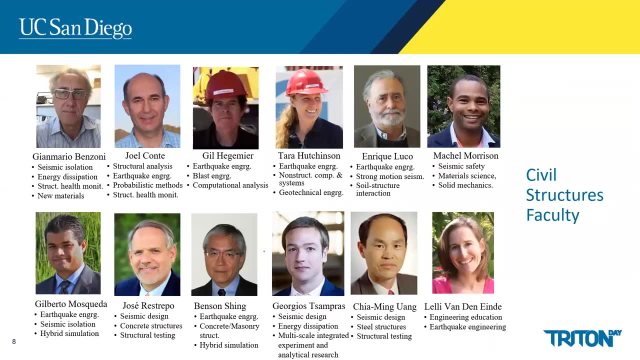 and test a complete geotechnical structural system. We also offer various classes that could be taken as part of technical electives that focus on the design of wood, pre-stressed concrete or steel structures, including seismic design detailing. Why UC San Diego? Well, our program is composed of several courses. 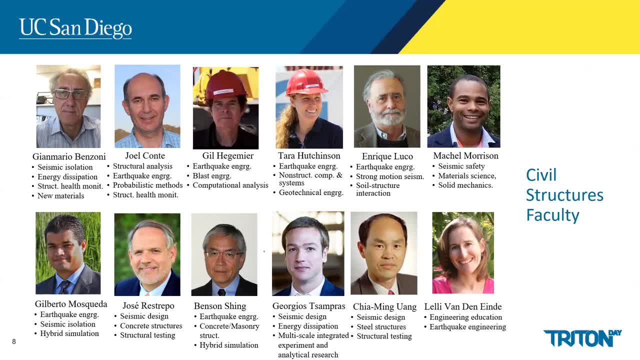 We have some of the best faculty in this area. in this area of civil structures, We have 12 world-renowned faculty that teach our undergraduate classes and mentor our students. As you can see, we have a very diverse faculty having specialties in steel structures, concrete. 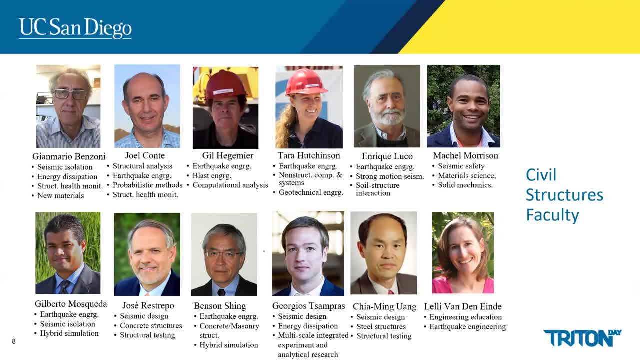 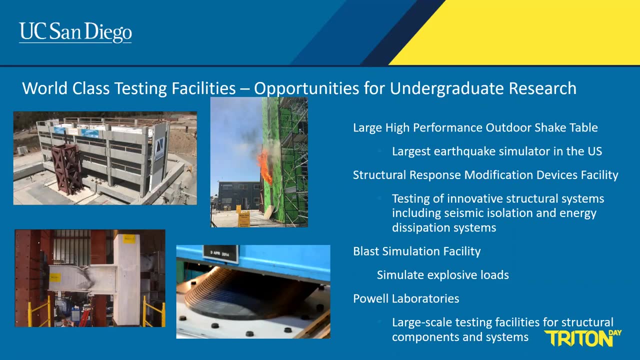 structures, masonry structures and other areas related to civil structures. At times we may have leading experts from practice teach design classes to build a stronger connection with the industry. Another important factor to consider is that at UCSD we have some of the most advanced laboratory capabilities available. in civil structures We test large-scale 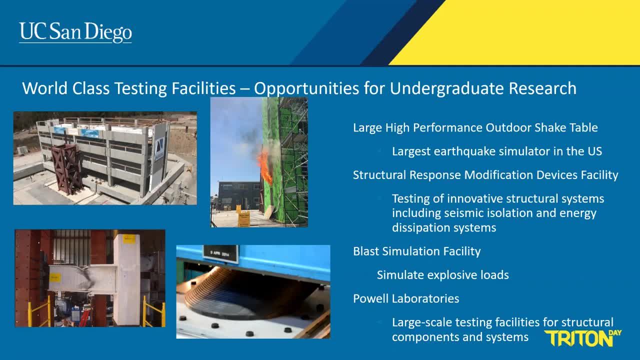 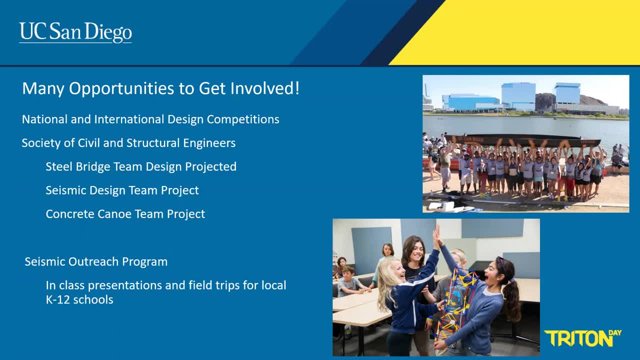